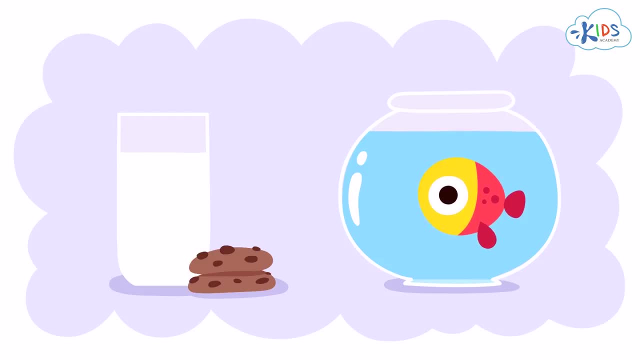 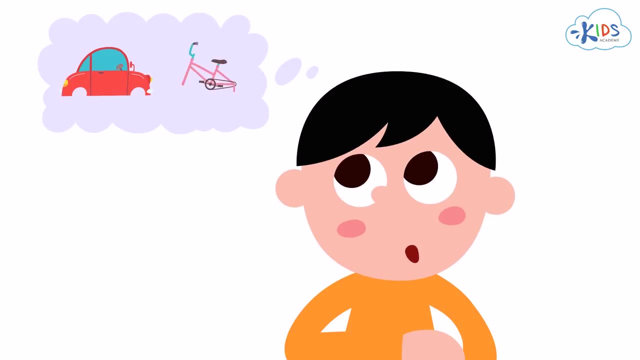 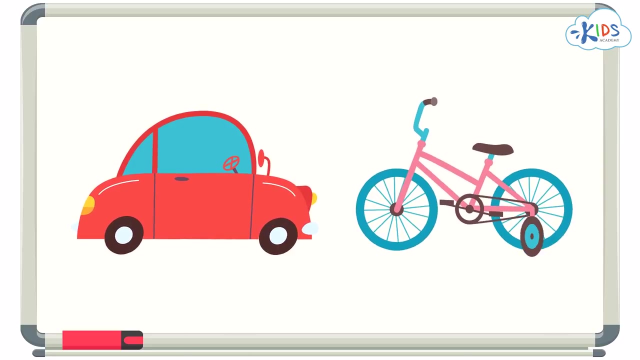 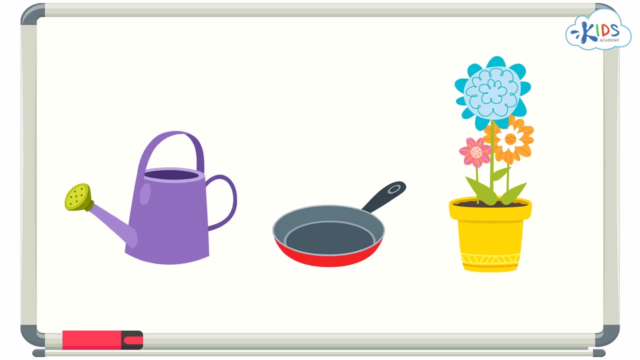 in water. Can you think of any other objects that fit together? Can you imagine a car or a bicycle without wheels? That doesn't look right. Wheels fit together with cars and bicycles. They belong together. How about these objects? Which ones fit together? Let's take a closer look at each object. The first object looks like something. 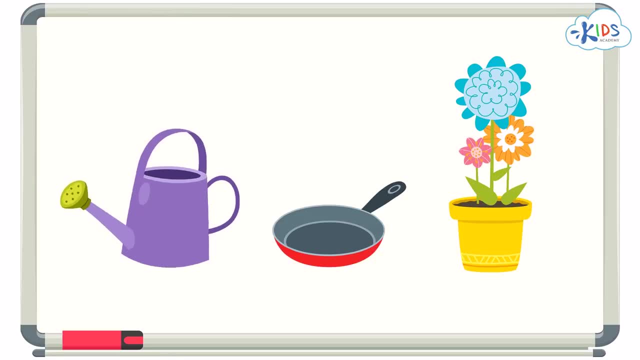 you use to water flowers or plants. The second object looks like something you use to water flowers or plants. The third object looks like something you use to water plants. The fourth object looks like something you use to water plants. The fifth object looks like something you use when cooking. 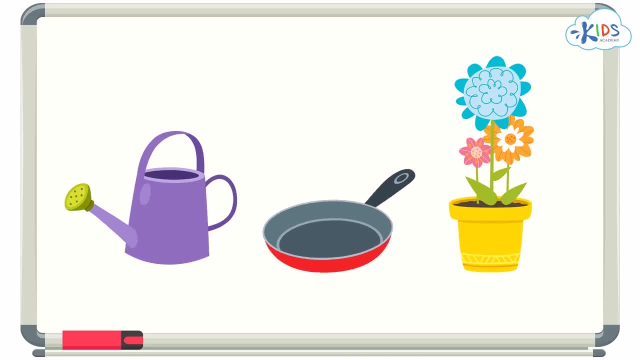 Hmmm, Do those objects go together? I can't see how. Let's look at the last object. These are some beautiful flowers. Do any of the other objects fit together with the flowers? Which objects belong together, like cookies and milk, The watering can and the flowers? 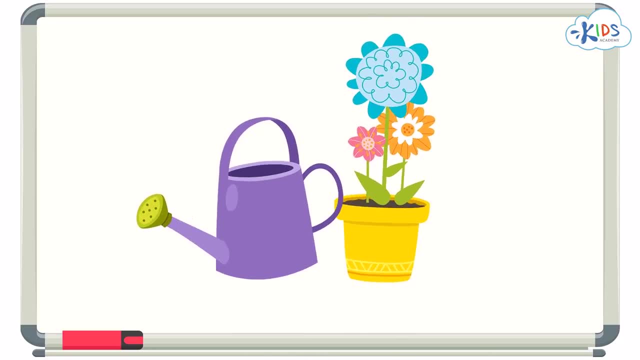 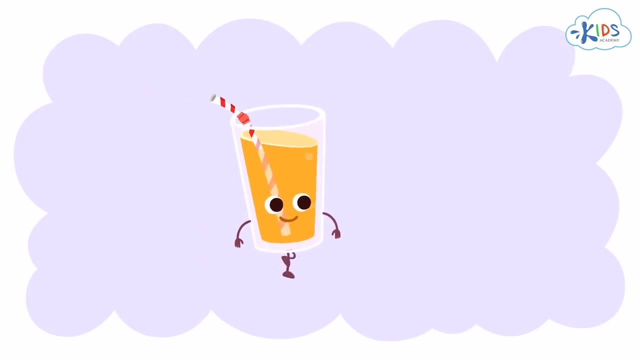 together. You can use the watering can to give the flowers water. That's how the objects fit together. There are so many ways that objects can fit or go together. I'll leave you with a challenge. What do you see? That's a glass of orange juice. Which one of these 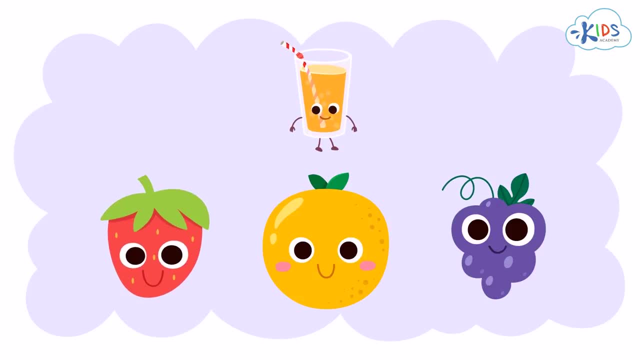 fruits go together with the orange juice. We have a strawberry, an orange and grapes. Which fits together best with the orange juice? I'll give you some time to think, but if you need more time you can pause the video and answer when you're ready. 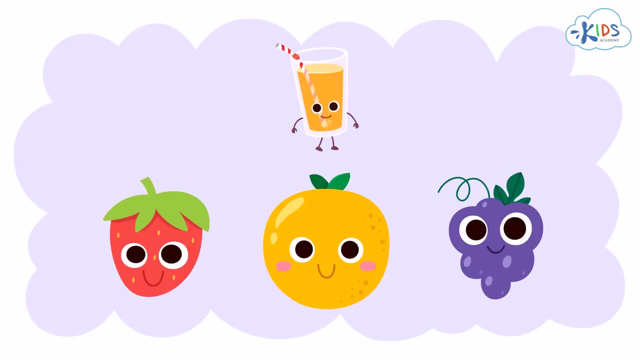 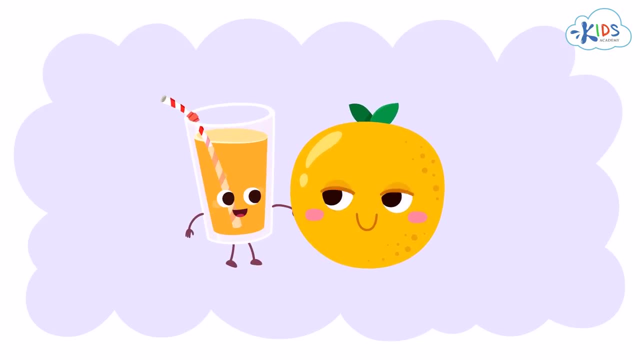 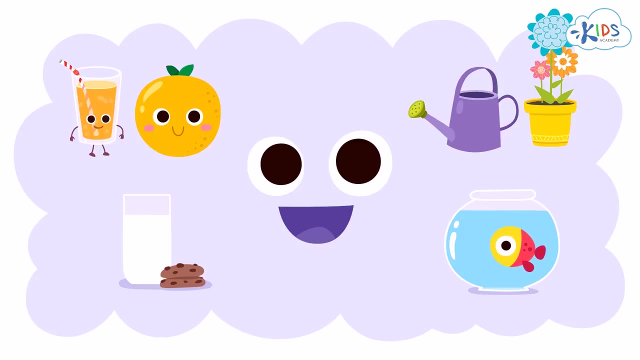 Okay, here's the answer. Well, it must be the orange juice, Because you can make orange juice from oranges. Those two objects fit together perfectly. Remember to first use your eyes to see if objects fit together. If you can't figure it out, think a little deeper and ask yourself: do these objects belong together? 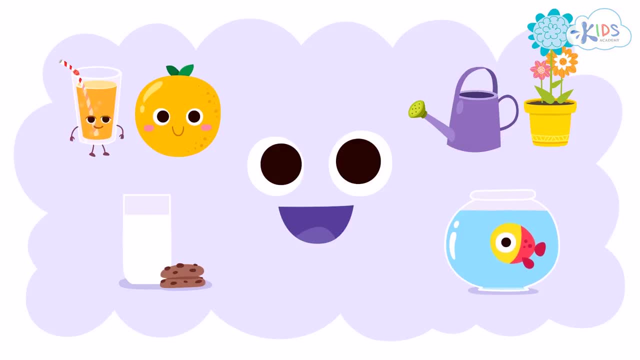 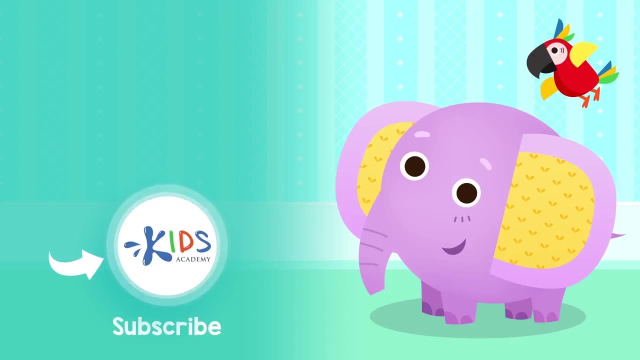 Thanks for watching boys and girls and we'll see you next time. Bye-bye.